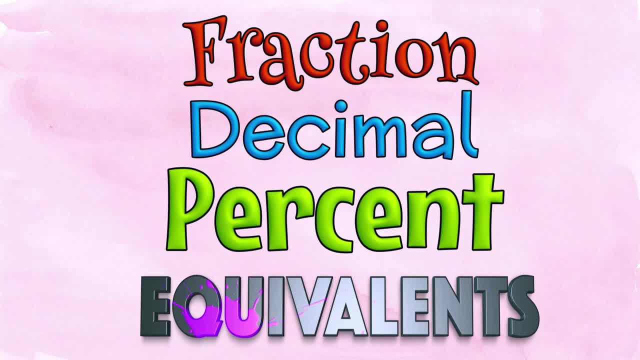 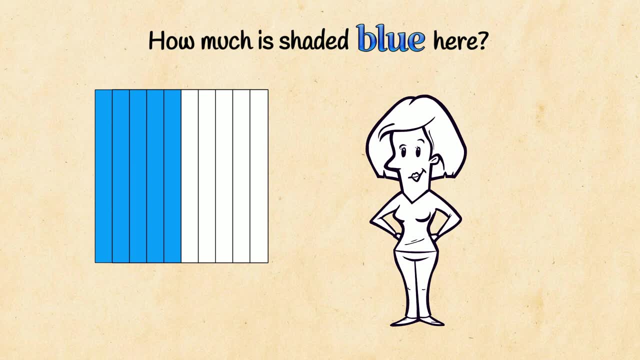 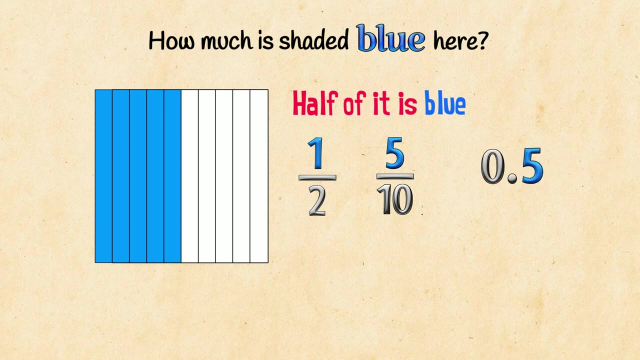 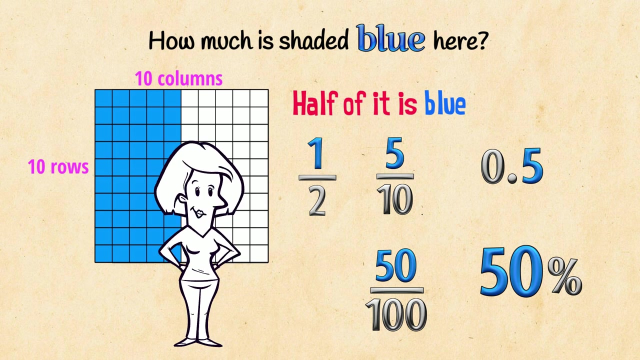 Fraction, Decimal and Percent Equivalents. 50 parts out of 100 are blue, And maybe you even said 50%. All these answers are correct. They're all equivalent amounts, Just different ways of showing the same information: Fractions, Decimals and Percents. 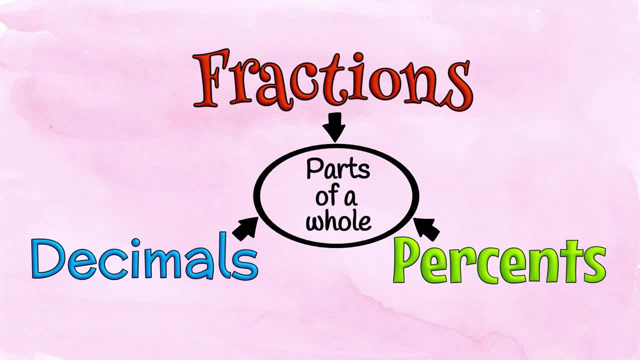 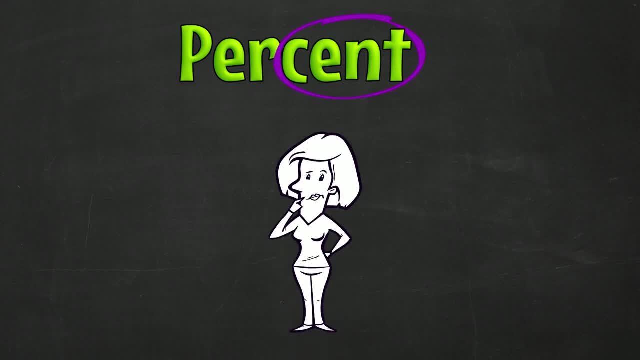 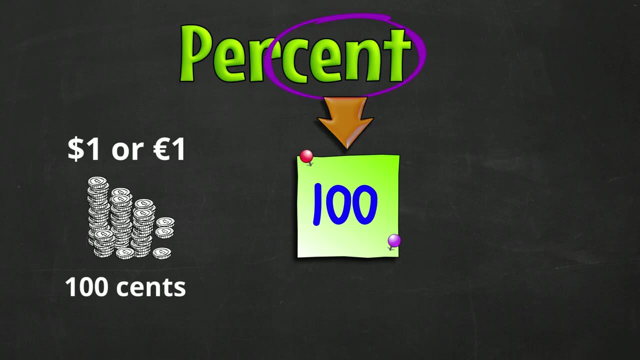 are all ways of showing parts of a whole. Percent might be a new term to you. Notice the word SENT in there. We know that 1 dollar or 1 euro has 100 cents. This is the percent sign. There's always some number attached to it. 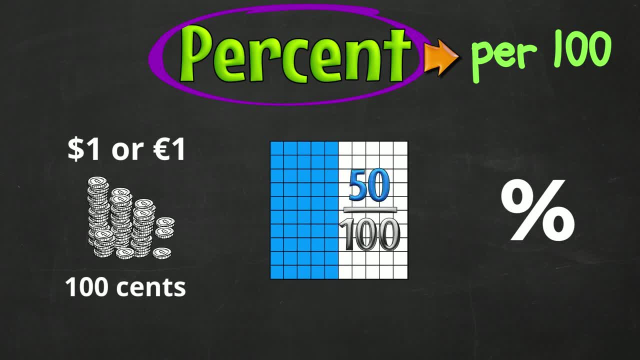 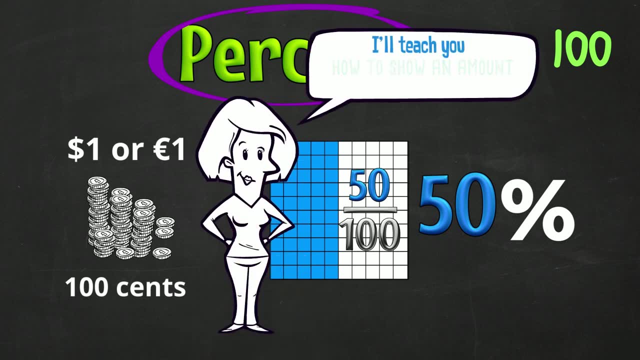 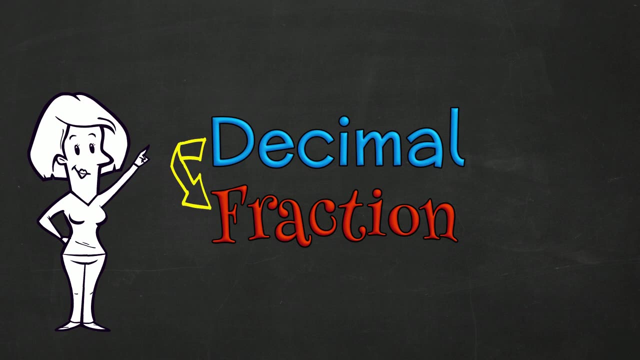 Like in our diagram, 50 parts out of 100 are shaded. It's 50% blue. Today, I'll teach you how to show an amount as a percentage. You already know how to switch from a decimal to a fraction and from a fraction to a decimal. 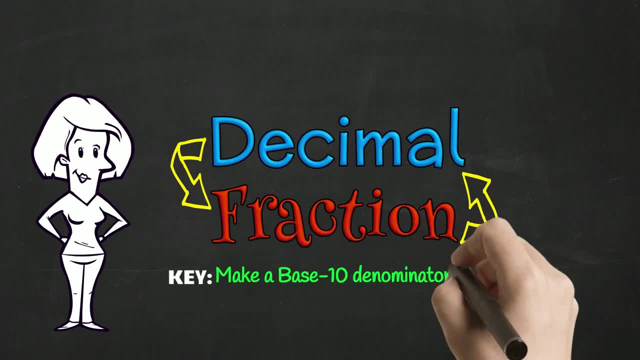 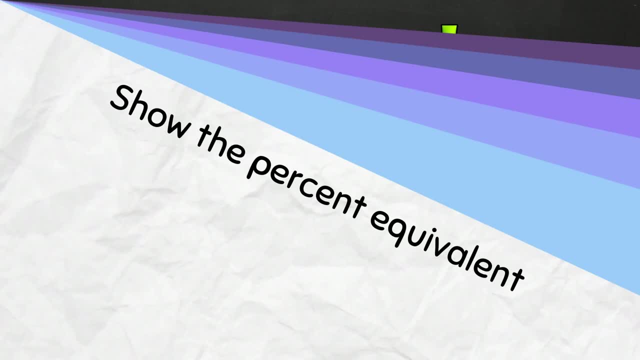 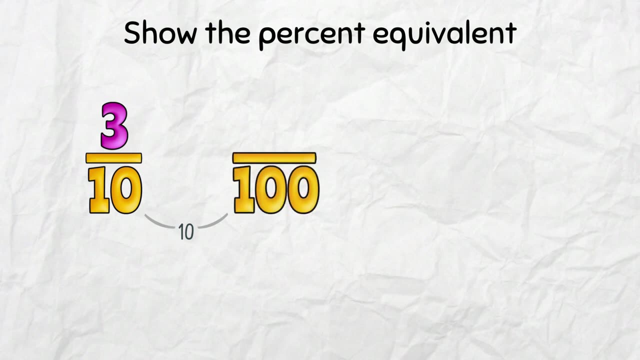 The key is in making a base 10 denominator, And if you can make a decimal, then finding the percent equivalent is easy. I have to show this as a percent. If I use a factor of 10, I get a denominator of 100 and a numerator of 30.. 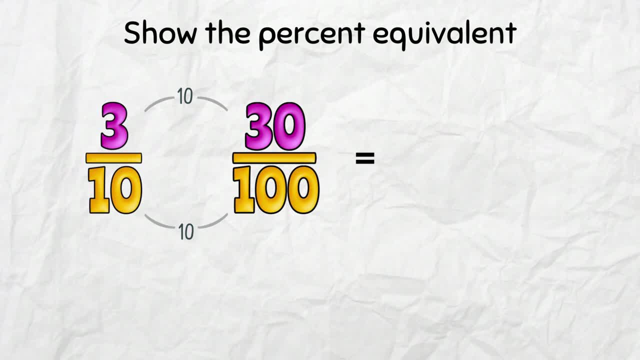 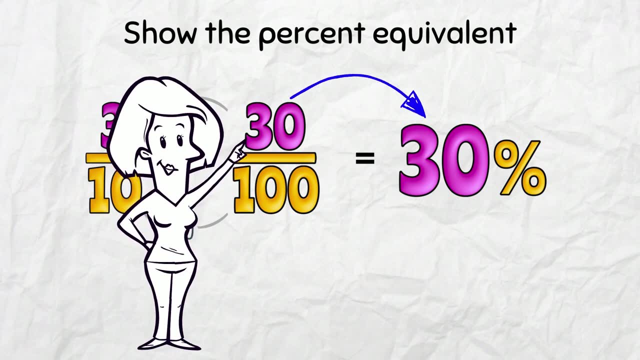 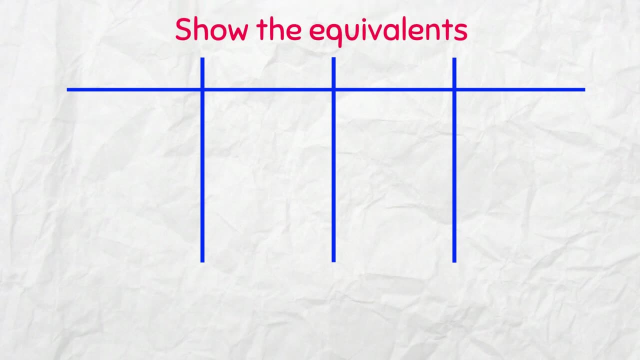 30 parts per 100.. Per 100 equals 30%. If I have a denominator of 100, then the numerator IS the percentage amount. Easy, Now we have to complete a table of equivalents. Here's a diagram and we have to show the equivalent. 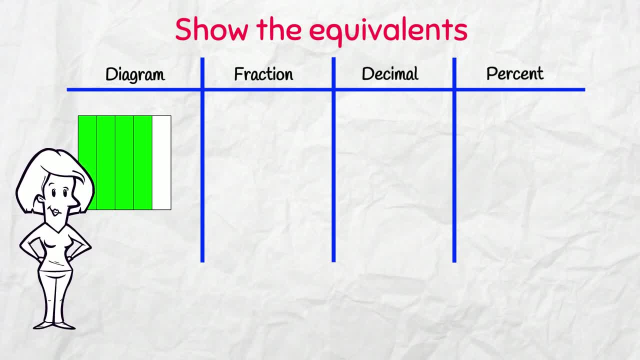 fraction, decimal and percent amounts. The diagram has 5 columns. 4 are green, that's easy. 4 fifths. Now for the decimal. I need a base 10 denominator for that. In fact, this table would be better. 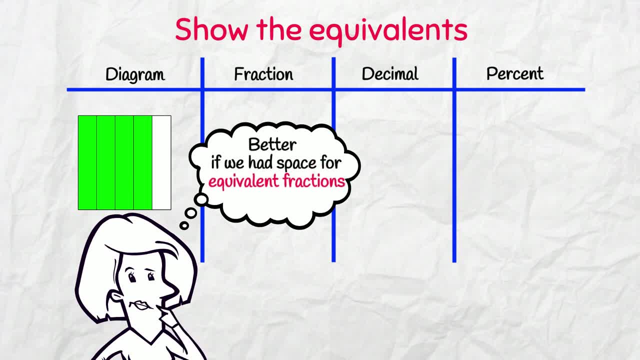 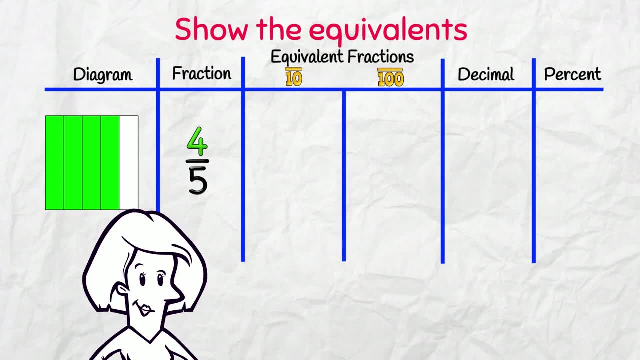 if we also had a space for equivalent fractions with a denominator of 10 and 100.. Let's do that now. That's better. Now let's make those equivalents. A factor of 2 gets me 8 tenths, And a factor of 10 gets me 80 over 100.. 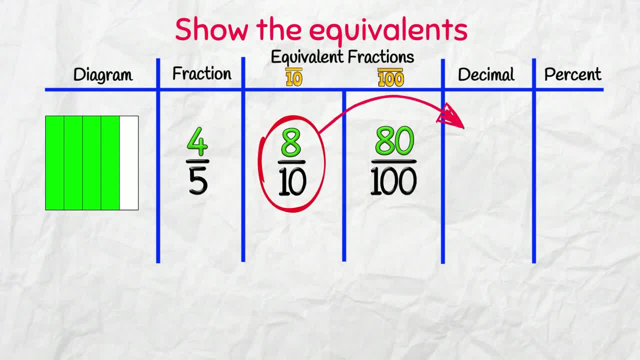 And a factor of 10 gets me 80 over 100.. For the decimal, it's 80 over 100.. For the decimal, 8 tenths is 0.8.. And for the percentage I need that denominator of 100.. 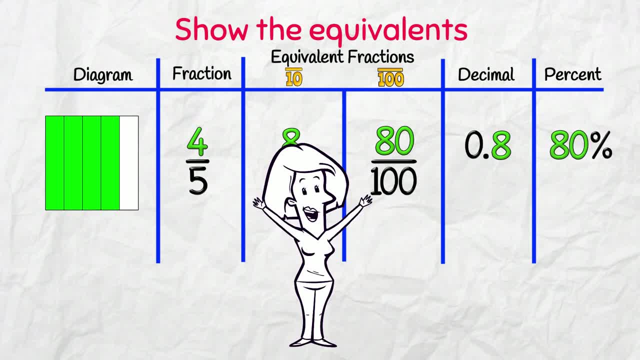 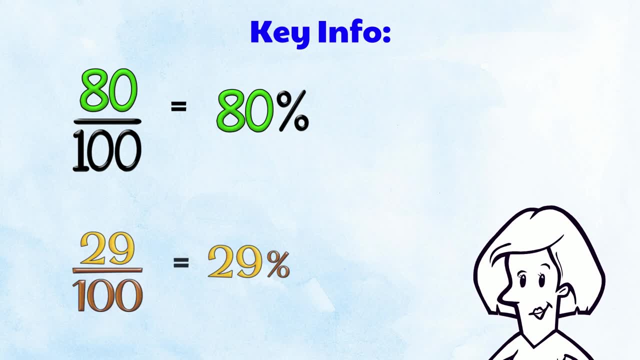 80 over 100 equals 80%. A number over a denominator of 100 equals the percentage amount. This is super important math thinking, and you're going to use it frequently. Let's do one more and then it will be your turn. This one's a bit different. 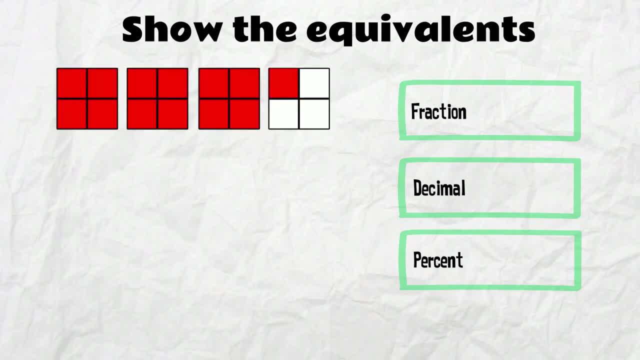 We've got 3 whole ones and 1 quarter red. You know how to show this as a fraction. It's a mixed number: 3 and a quarter. What about the decimal equivalent? 3 whole ones, point and then the quarter. 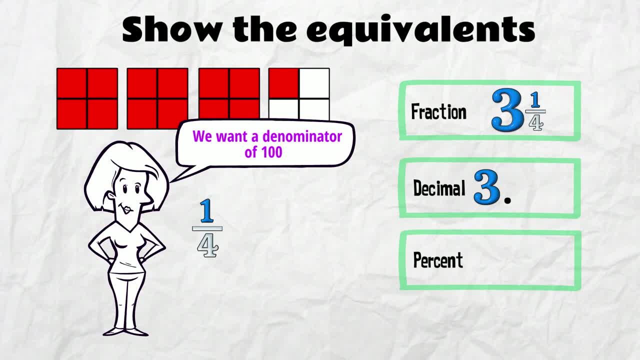 Well, we want a denominator of 100.. Multiply by 25.. Same up. top 25 over 100.. The decimal part is 0.25.. 3 and 1 quarter equals 3.25.. 0.25 as a decimal. 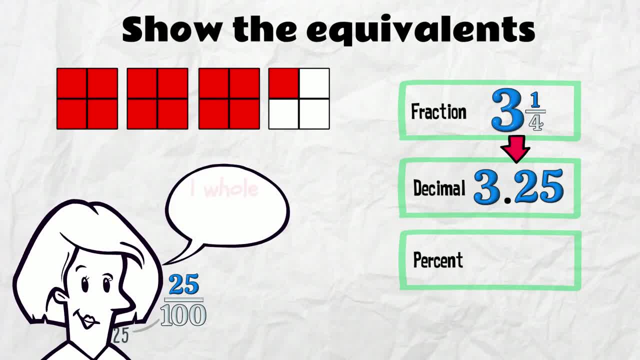 Now, how about that percentage equivalent? We know that one whole is worth 100%. That means this is 100%, and this is 100%, and so is this, And here we've got 1 quarter, which we know is 25 over 100. 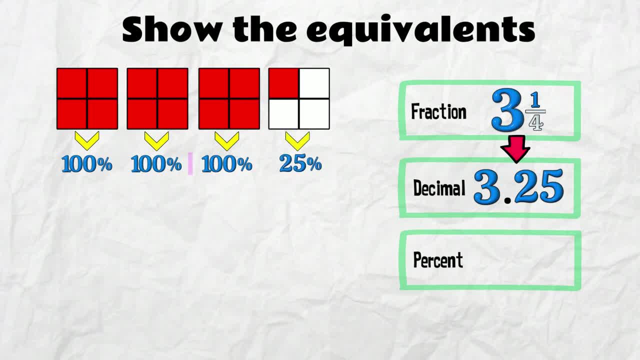 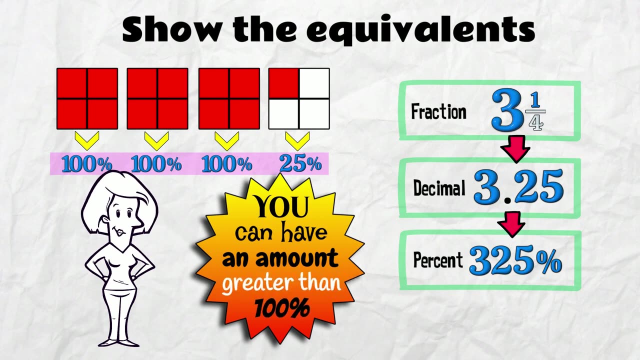 or 25%. If we count these up, you'll see that we have 100,, 200,, 300, and 25%. Get this. We've just proved you can have an amount greater than 100%. Possibly a bit mind-blowing.